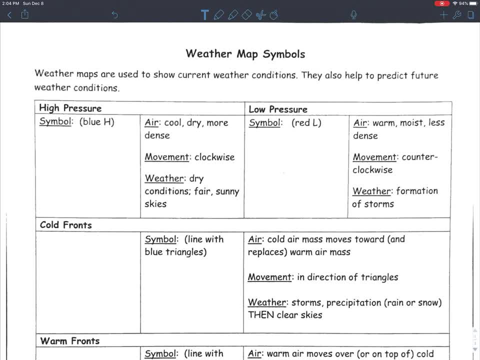 familiar. This is what we talked about when we talked about wind. So when we look at high pressure, our symbol for high pressure is a blue H. So I'm going to go ahead and draw a blue H in here, Because remember that high pressure is a big blue H, So we're going to see that blue H on a weather. 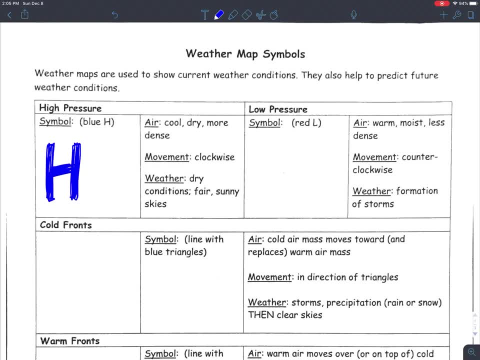 map. One thing that you might want to remember about high pressure is: high pressure is what we call happy weather. So I'm going to write happy, I'm going to draw a little smiley face. What do you think happy weather would be? Yeah, if you said sunny weather. 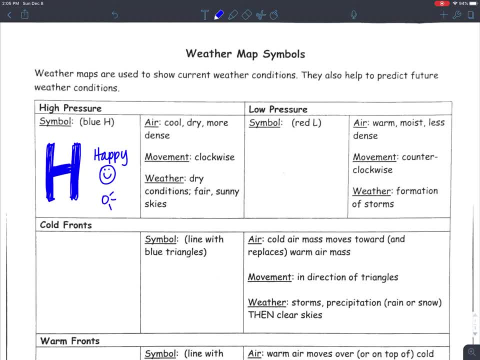 happy weather is what we think of as sunny weather. So I'm going to draw a little sun here to remind myself that high pressure is happy weather. Go ahead and grab your highlighter. We're going to highlight the word high pressure. I'm going to highlight where it says blue H, so that I can remember that. Let me actually make. 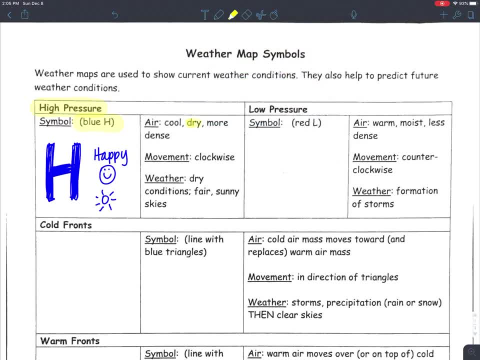 this a little smaller. Okay, I'm going to highlight that the air is dry. Remember that the weather for today is fair, sunny skies. So when we say dry conditions, we mean no rain. So high pressure is a blue H. The air is dry, which means we have fair, sunny skies. Let's look at low pressure: Low. 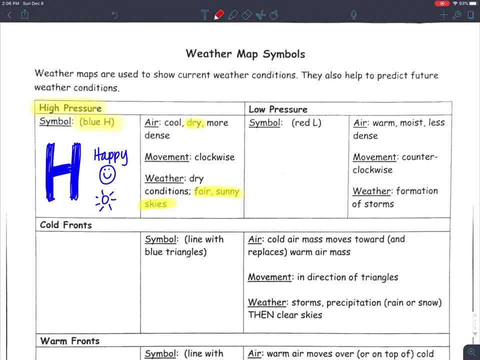 pressure was something we also talked about when we talked about winds. I'm going to grab my red color. Remember that low pressure is represented by a red L. So I'm going to draw a big red L here. pressure is represented by a red L. An easy way to remember low pressure is: low pressure is lousy. 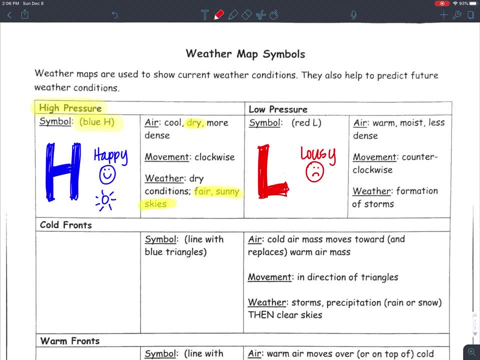 weather, So I'm going to draw a sad face. Lousy means not that good. It's not good weather. What kind of weather do you think would be lousy weather? Good, rainy weather? So I'm going to draw a cloud here with some rain. So low pressure is lousy weather, It's going to be rainy weather. 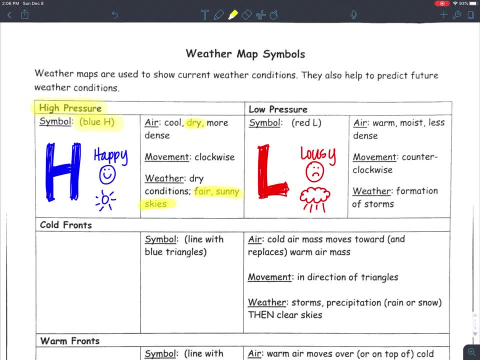 Go ahead and grab your highlighter, Highlight the words low pressure. We're going to highlight that it is a red L And we're going to highlight the word moist here. When air is moist, it means there's a lot of moisture in the air, It means the air is really. 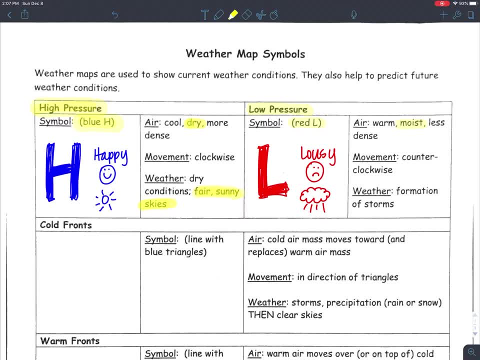 wet, which allows for precipitation or rain. So that's why we typically see, with low pressure, we see storms forming. So go ahead and highlight formation of storms. So because the low pressure air, the air tends to be wet, that's why we see storms In high. 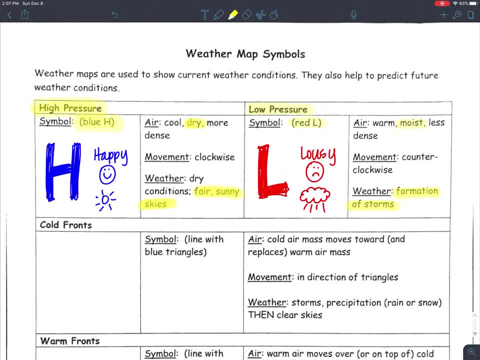 pressure, the air tends to be dry, So we see sunny skies, not a lot of clouds, not a lot of rain. The next thing we're going to look at is fronts like cold fronts and warm fronts, And I want you to grab your pen or pencil and we're going to write something down here at the top of our page. 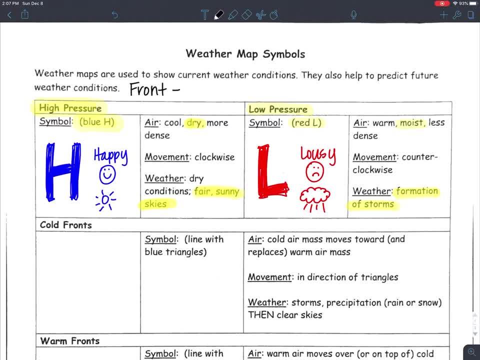 Okay, we need to know what a front is. So we talk about a cold front or a warm front. A front is just a boundary between two air masses. A boundary between two air masses? Okay, so this could mean a boundary between cold. 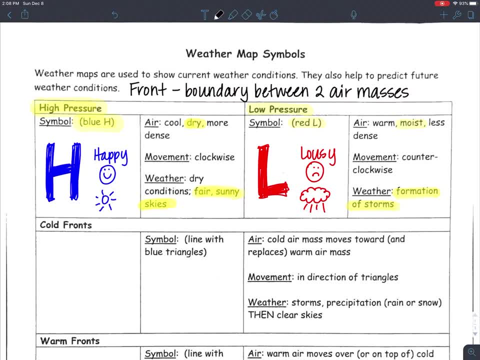 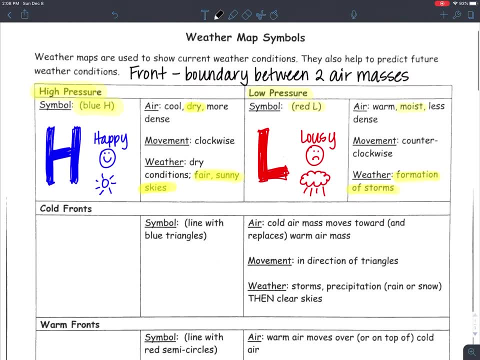 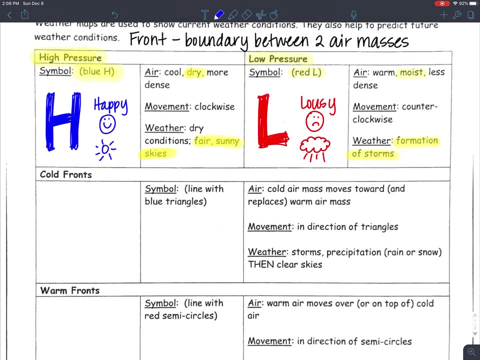 dry air and warm, moist air. Okay, so it's just the boundary between where two different types of air meet. So the first thing we're going to look at is our cold front. So I'm going to grab my blue color and it says that our cold front symbol is a line with blue triangles. So I'm going to draw a line. 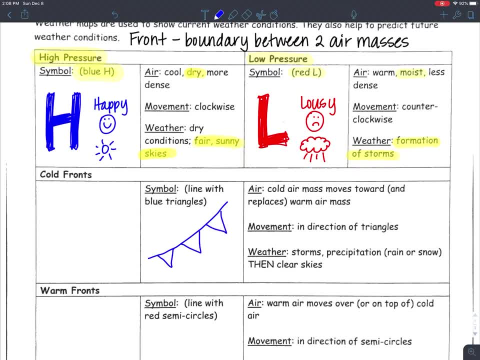 here. You guys have probably seen something that looks like this before. Okay, this is going to be my cold front. It's a line with blue triangles. I always remember it because it kind of looks like icicles. So cold front- icicles are cold. It's a line with blue triangles. 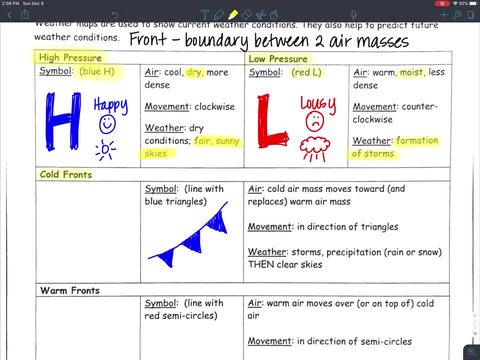 So go ahead and grab your highlighter. We're going to highlight the word cold front, We're going to highlight line with blue triangles And we're going to highlight the weather that is associated with cold fronts. That's going to be storms and precipitation, then clear skies. 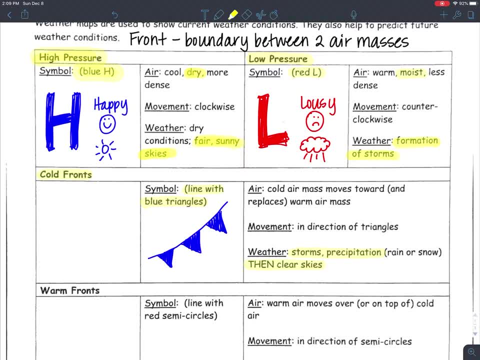 So storms and precipitation, then clear skies. So typically what we see is, as the front is approaching, as it's moving towards us, it's going to be really stormy and rainy, A lot of clouds, a lot of rain. But as that front pushes, 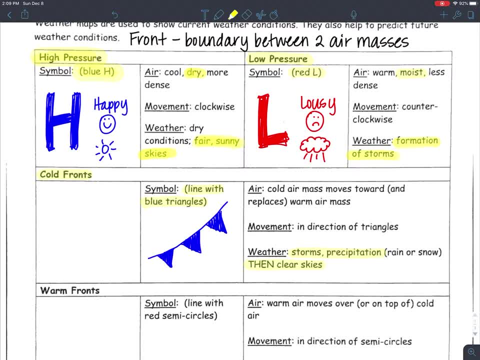 through. there's going to be cold air, typically behind that front, And that cold air is that sinking air, And that sinking air allows for really, really, really sunny, clear skies. So it's going to be precipitation and then it's going to be clear skies. 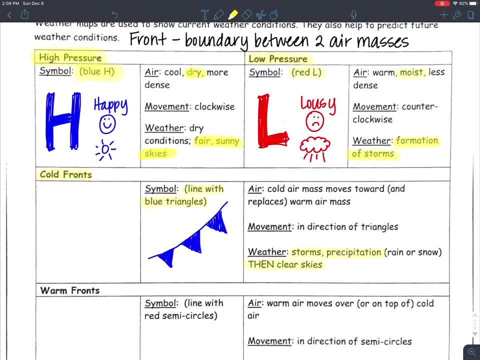 One thing you also have to know is the movement of the front. So in this case in particular, the movement is going to be where the triangles are pointing. So if we had to look at this and let's say we had north east, 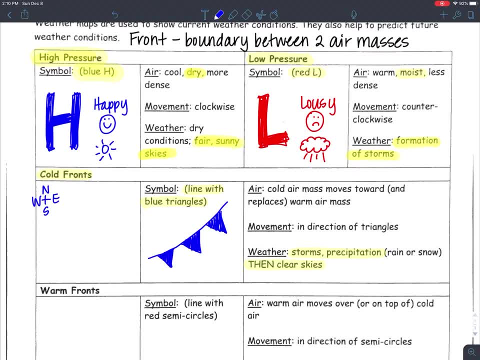 south west. Okay, here's our compass. Which way would this particular front be pointing? Which way would this particular front be pointing? Which way would this particular front be moving? Good, If you said south east, you are correct. This front would be moving south east. 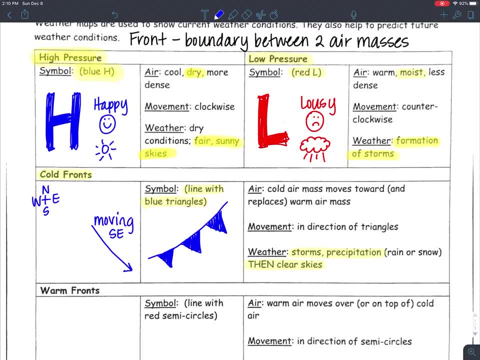 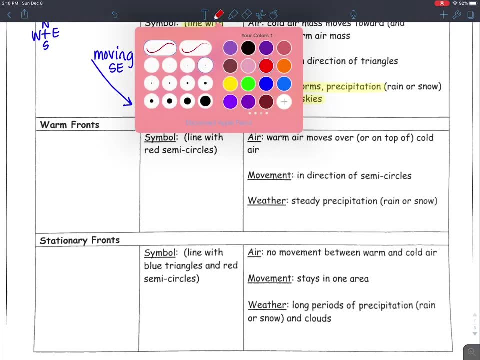 I'm going to write moving south east right, because those triangles are pointed towards the south east. All right, let's talk about warm fronts next. I'm going to grab my red color for this. Warm fronts are represented by a line with red semicircles. 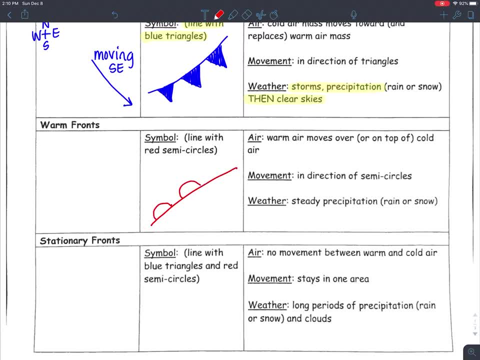 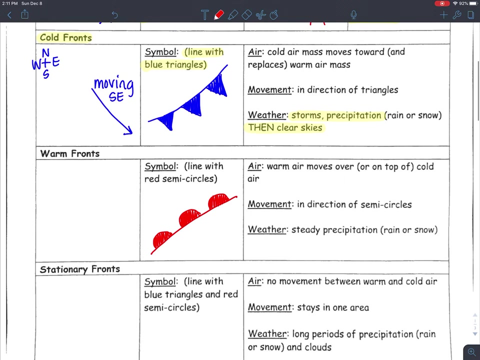 So I'm going to draw a line here and I'm going to draw some half circles. Semicircles means half circles that are red, like this. All right, Let's grab our highlighter. We're going to highlight warm fronts. We're going to highlight line with red semicircles. 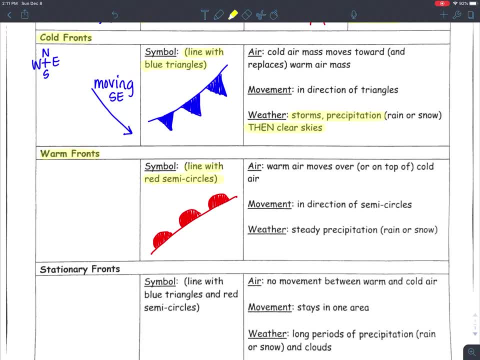 I always remember that warm front is the red half circles, because they kind of look like half suns And the sun is warm. So that's how I remember that the half circles that are red are warm fronts. Here we have steady precipitation, So I want you to highlight steady precipitation. 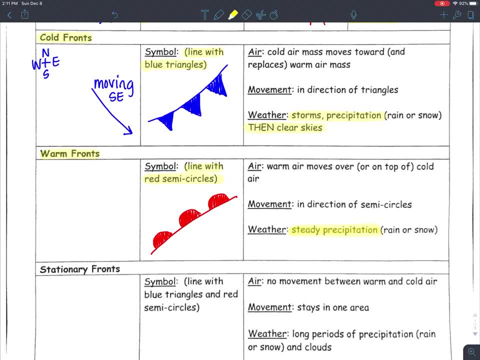 That means, as the sun is moving through, it's going to just rain a lot. It's just going to rain steadily. It may not have a lot of big storms, but it is going to rain quite a bit. So I want you now to look at the direction that this is going. 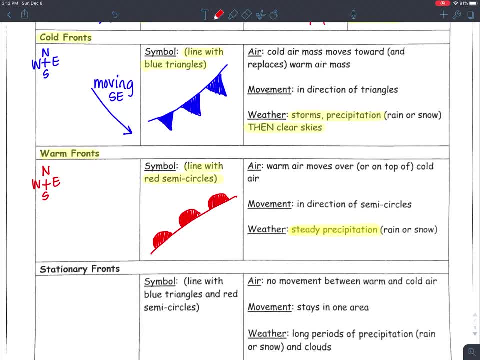 So I'm going to write my compass here again- north east, south west- And now I'm going to look at the direction of the semicircles to determine where this particular front is going. So which direction do you think the front is moving? 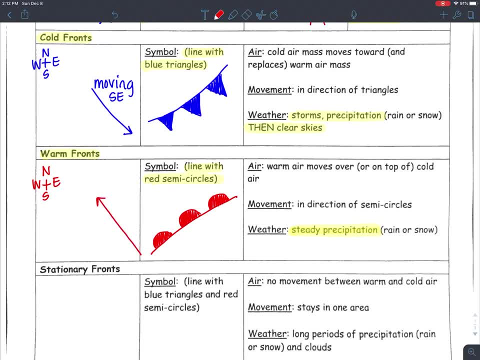 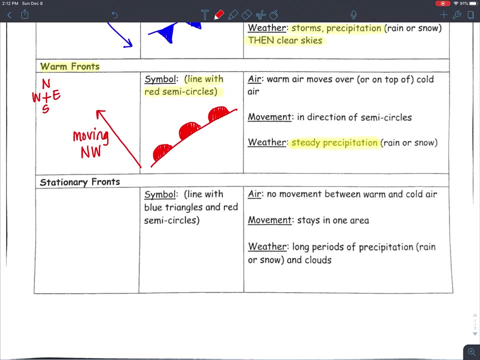 If it looks like this, Good, It's going to be moving north west, Excellent. Let's talk about stationary fronts. Stationary front is a line with blue triangles and red semicircles. Blue triangles and red semicircles. So I'm going to grab both colors here and I'm going to draw a blue triangle. 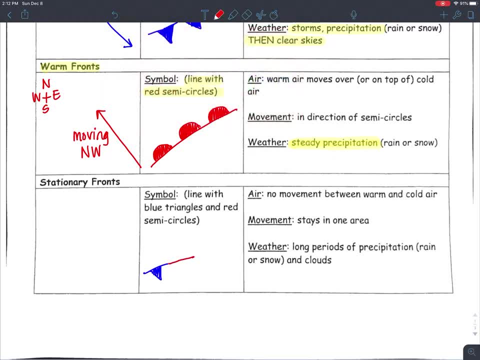 Like this, And then a red semicircle like this, and they alternate every other one like this. So now I'm going to grab my highlighter, I'm going to highlight the word stationary front, I'm going to highlight line with blue triangles and red semicircles. 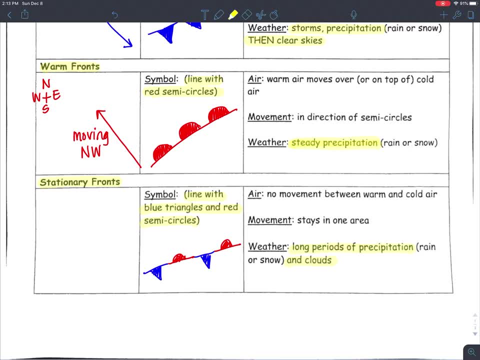 And I'm going to highlight long periods of precipitation and clouds. So when we see a stationary front, we're just going to have again raining clouds for a long period of time. Now, last thing, let's look at the movement of that stationary front. 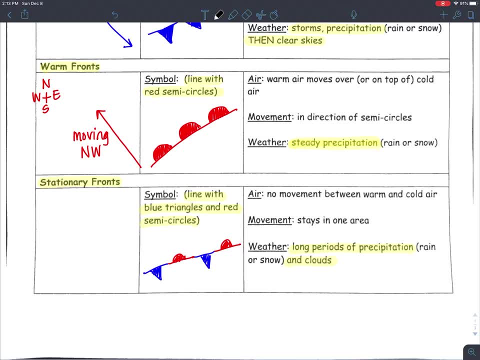 Which direction do you think the stationary front is going? Aha, trick question, If you know what the word stationary means. stationary means that it stays in one area, So stationary fronts are going to stay in place. They're going to stay in place. 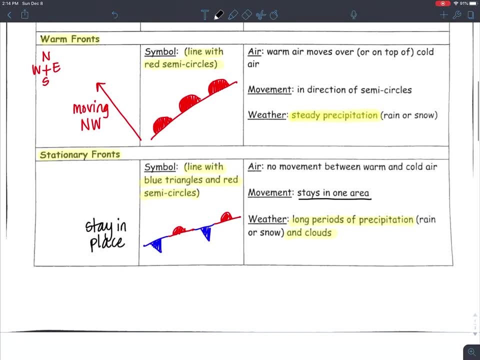 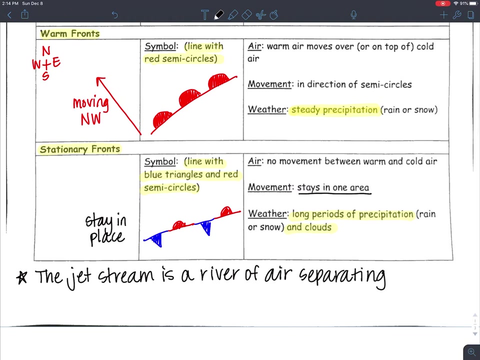 One last thing we're going to write down is the jet stream, and we do need to know the jet stream, So I want you to write this down. The jet stream Is a river of air high in the atmosphere, Separating Different air masses. 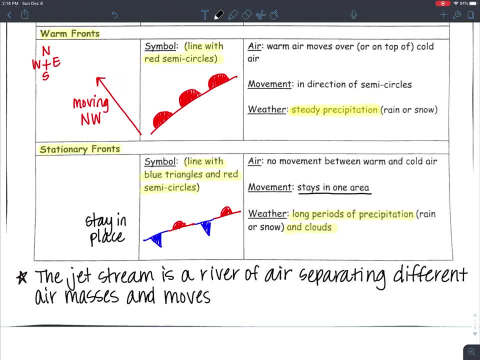 And moves From West To East. The jet stream is a river of air separating different air masses and moves from west to east, So the jet stream is also going to be responsible for what's moving some of the weather patterns that we see in the United States. 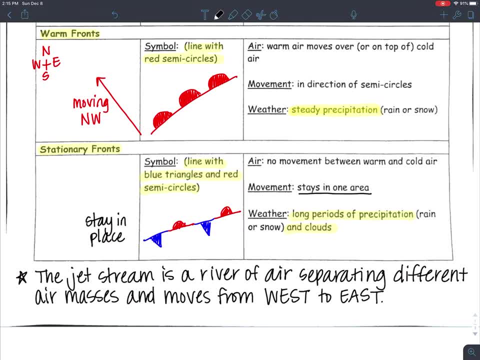 So most of the time, those weather patterns are going to be moving from the west to the east, Okay. so basically they would be going in this direction. Okay, across the United States. So I want you to grab your highlighter, I want you to highlight jet stream and I want you to highlight west to east. 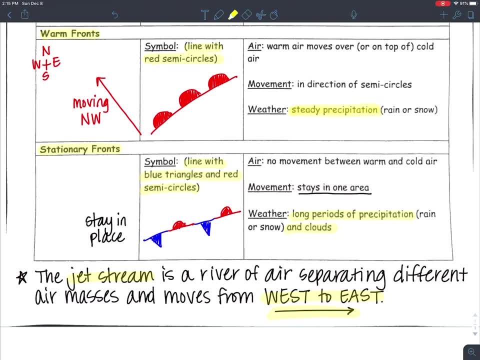 And you can even highlight this little arrow there. They're going from west to east And that is what you need to know and recognize about fronts and pressure. So, those weather symbols on a map, Let's go ahead and practice. I want you to turn your notes paper over to the back. 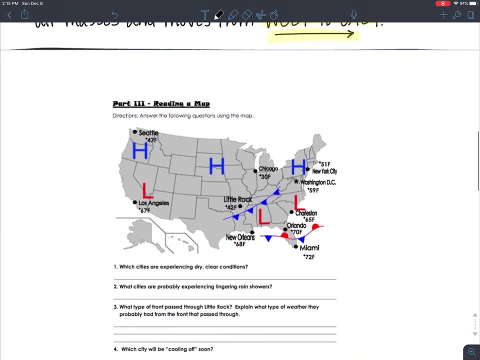 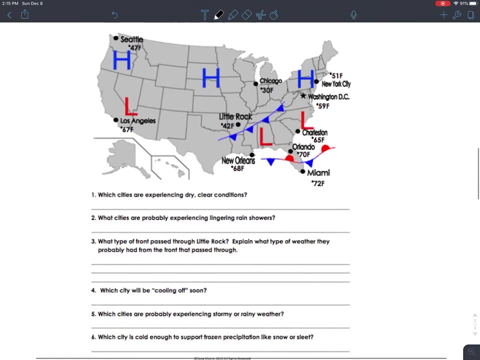 Turn your notes paper over to the left. Turn your notes paper over to the back And I want you to number one through six. Turn your notes paper over to the back And I want you to number one through six. I want you to pause the video. 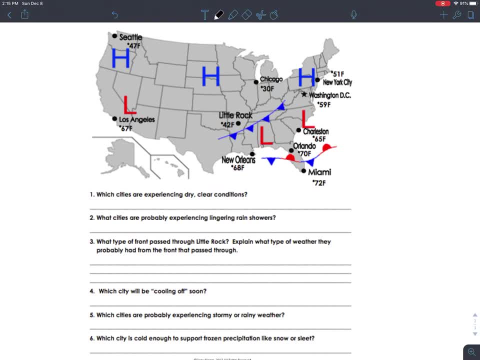 And I want you to write down the answers to questions one through six By reading the weather map that you see on the screen. So right now, pause the video, Answer questions one through six And then we will go over them, All right. 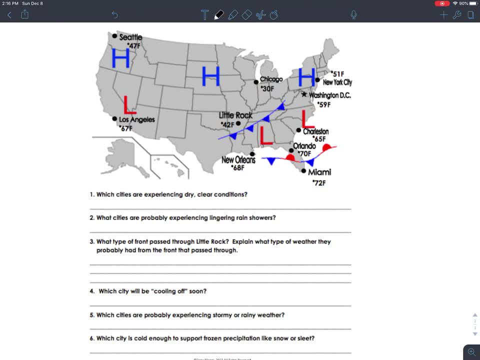 Let's go over your questions. Number one: Which cities are experiencing dry, clear conditions? So if I look at dry, clear conditions, what type of symbol am I going to be looking for? If you said the high pressure, the H, you are correct. 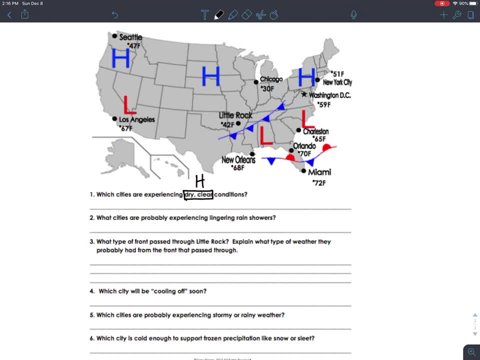 So which cities would be experiencing dry, clear conditions? Good, Seattle And New York City. Good. Number two, Which cities are probably experiencing lingering rain showers, Those showers that maybe are going to stay around for quite a bit of time, All right, 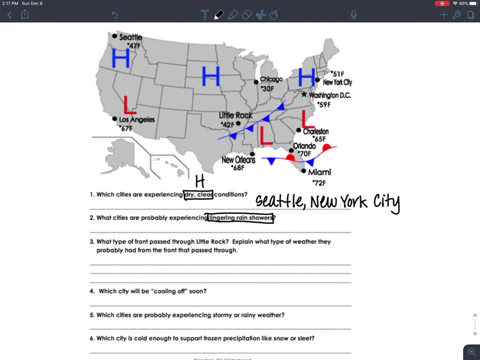 I want you to think about that. Good, If you said Orlando or Miami, you are correct. That's because we have this stationary front here. Remember that stationary front is lingering. Lingering means it's going to stick around for a while. 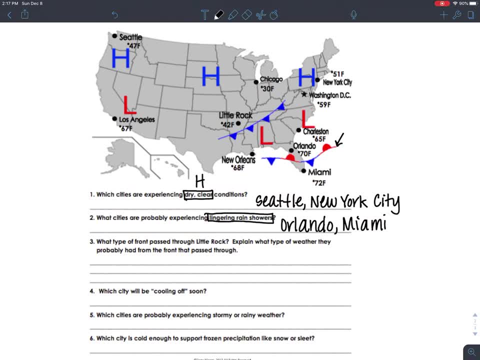 Number three: What type of front passed through Little Rock? So what was the name of that front that passed through Little Rock? Good, That was a cold front. Explain what type of weather they probably had from the front that passed through. So what kind of weather is associated with the cold front? 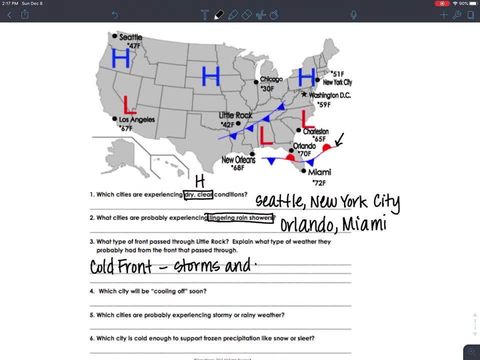 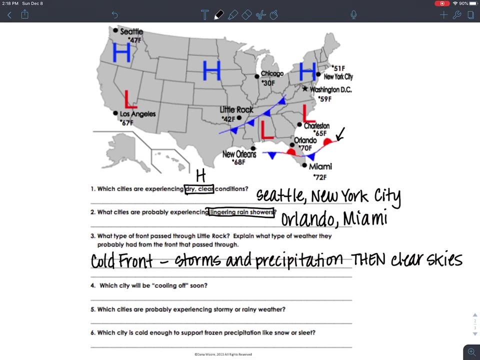 Good, so we can say: storms and precipitation, And then what would it be after those storms and precipitation leave? Good, then, clear skies, All right. number four: which city will be cooling off soon? So what would we look for if it's gonna be cooling off soon? 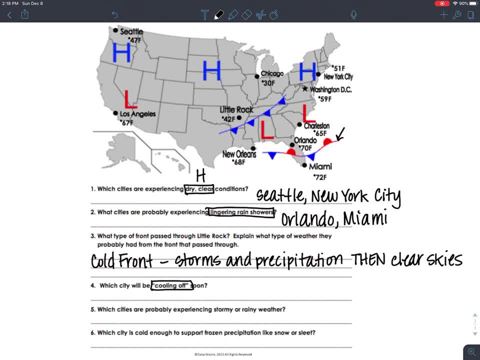 Good, we're gonna look for a cold front if we see cooling off. So which city is gonna have a cold front soon? Excellent, New Orleans. So that cold front is gonna be moving in this direction, so New Orleans would probably be the first city. 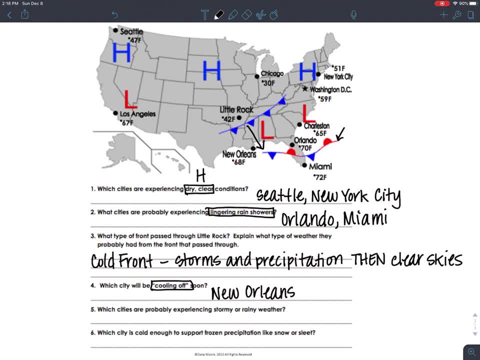 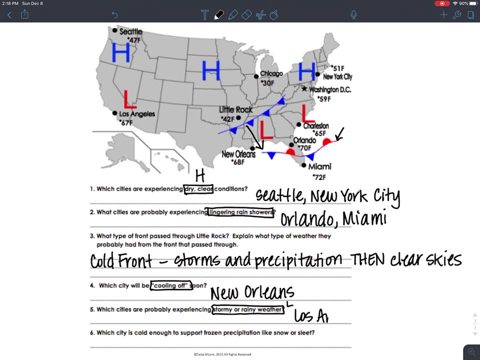 to experience that cold front Number five, which cities are probably experiencing stormy or rainy weather? So where would we see stormy or rainy weather? Good, we're gonna look for that low front. So I would say Los Angeles and Charleston. 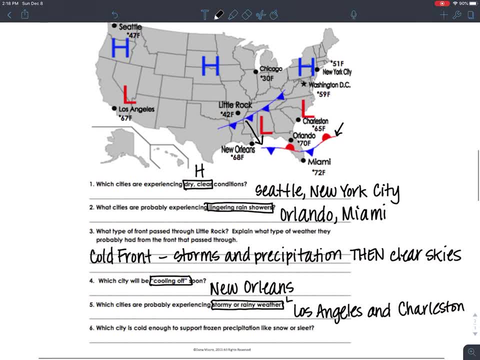 Both of those have a low pressure system. Number six: which city is cold enough to support frozen precipitation like snow or sleet? So I want you to look and see. It's gonna have to be below freezing in order to support that.